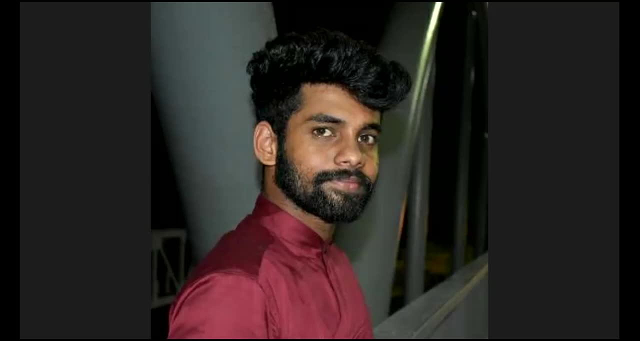 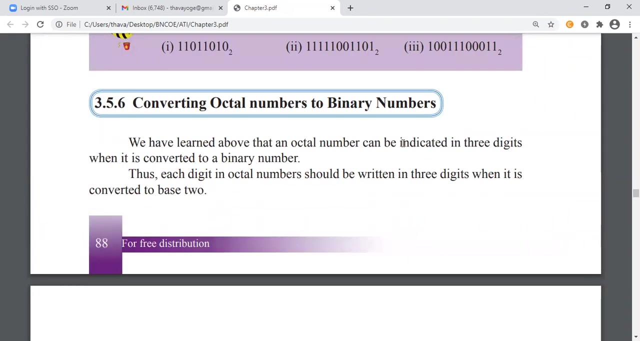 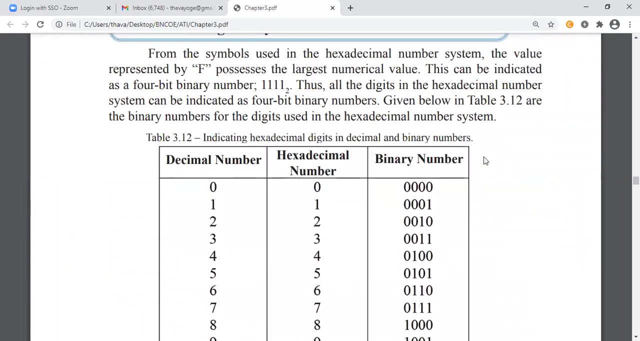 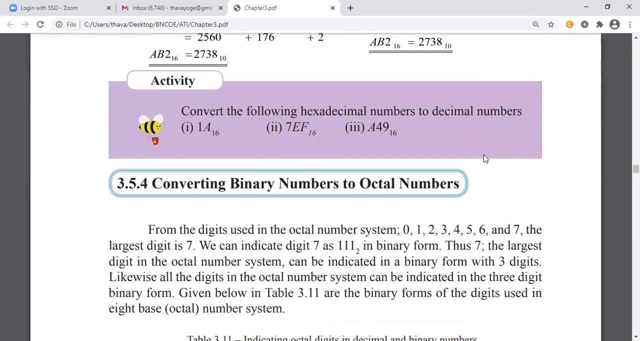 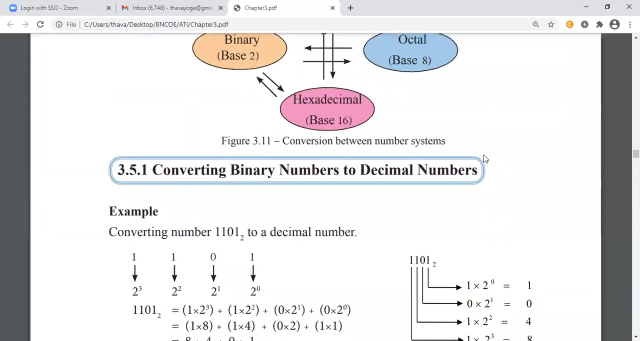 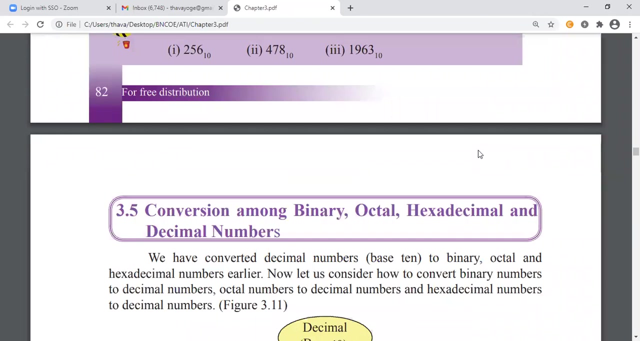 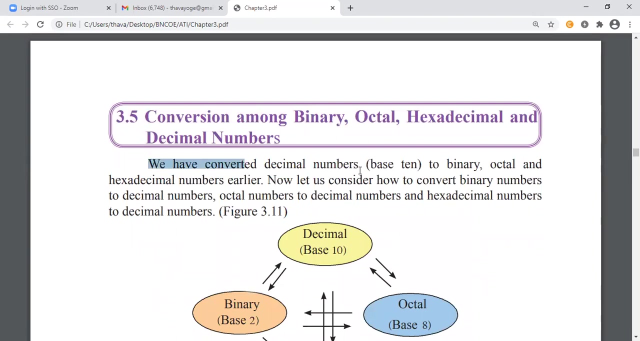 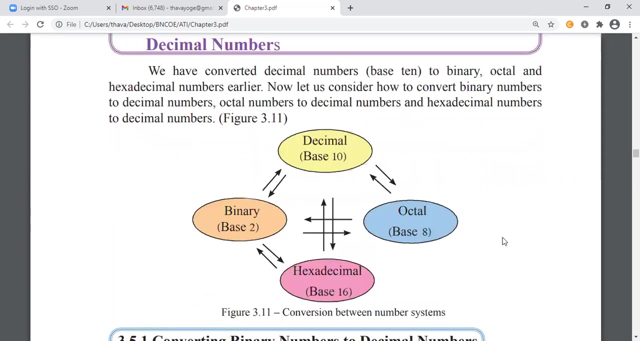 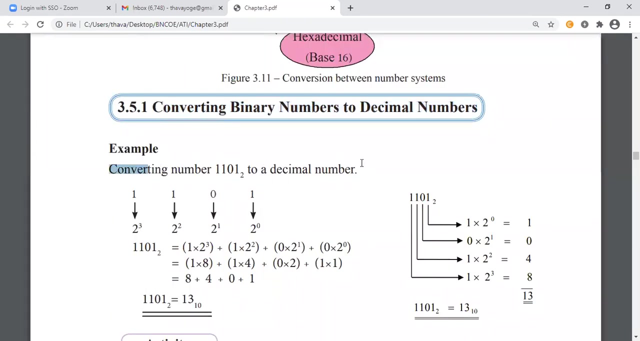 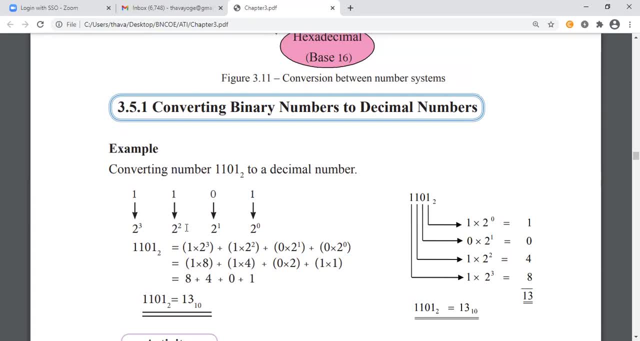 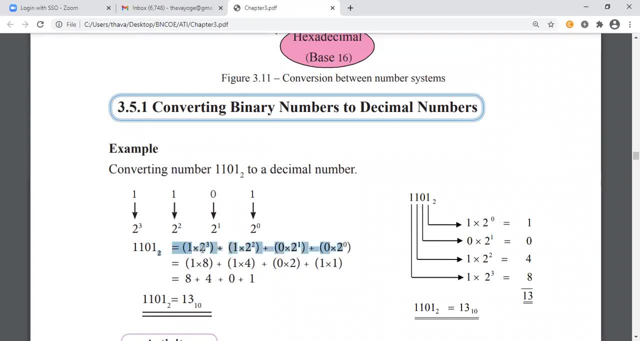 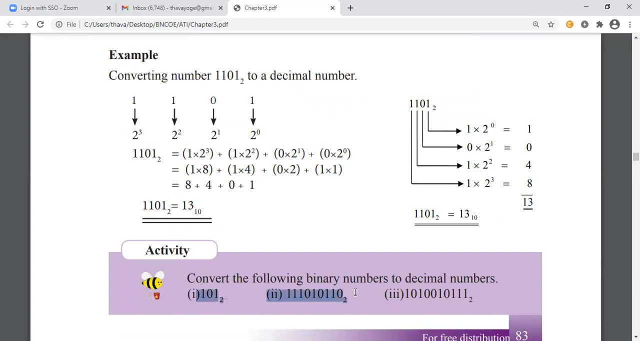 I will give you a bigger example. You know, the circumference of 2x2 is 8, right 2x2 is 4, 4x2 is 8.. This is an easy method. I will just write it down. 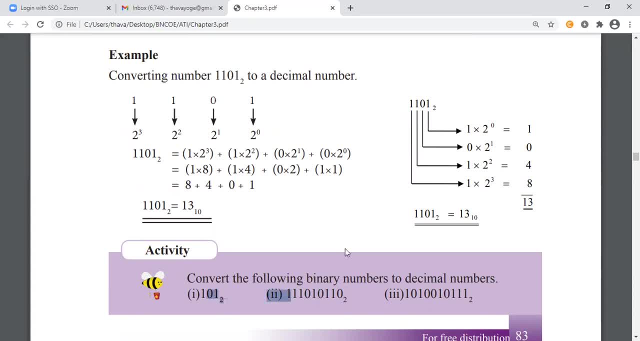 I will write 10x5,, 2x5,, 2x5,, 2x5.. I will convert the first number. I will do the same for the second number. It will be easy for you. Do the same for the third number. 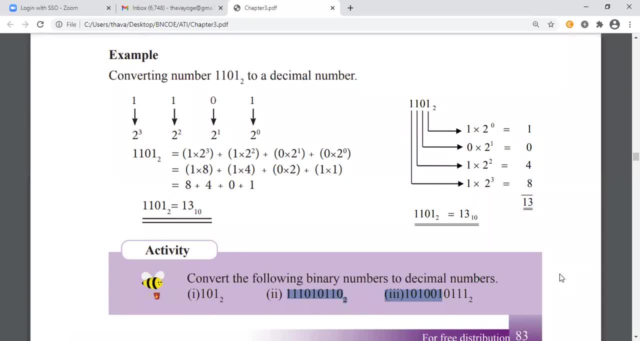 It will be easy for some. Some of you have become Beacons, right, Those who came from the Arts background or those who came from IT. I will do the same for them. For those who are not intelligent, I will do it later. 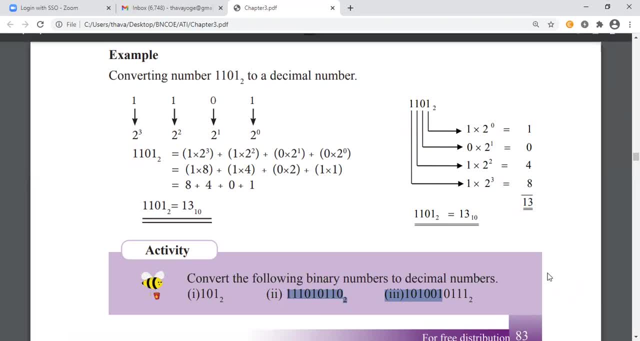 Do the same for the highlighted numbers. Don't do it alone. Do it on your own. I will write it down. I will say 3x4, 4x4, 2x4.. 3x4, 4x4.. 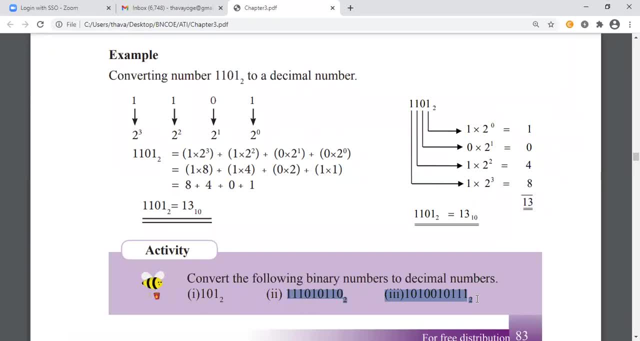 3x4, 4x4, 2x4.. 4x4, 4x4.. 4x4, 4x4, 2x4.. 4x4, 4x4.. 4x4, 4x4.. 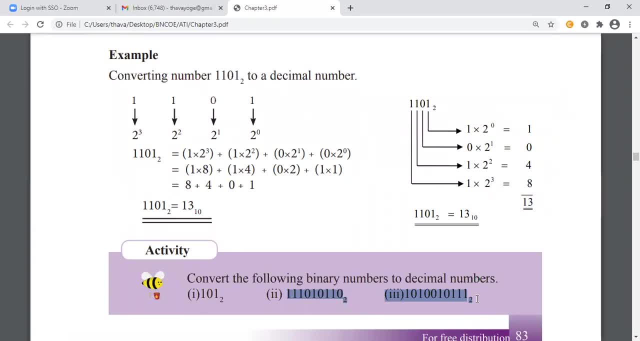